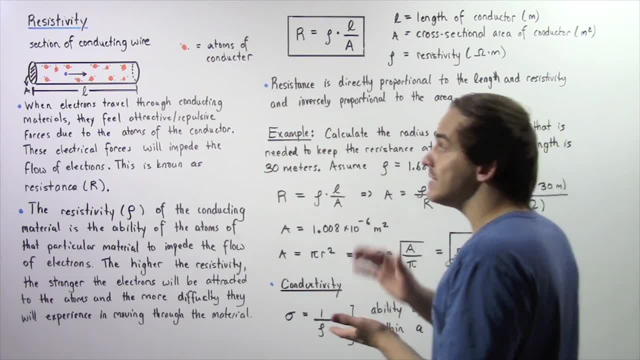 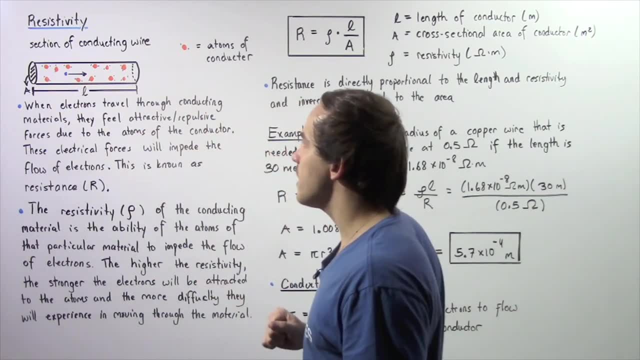 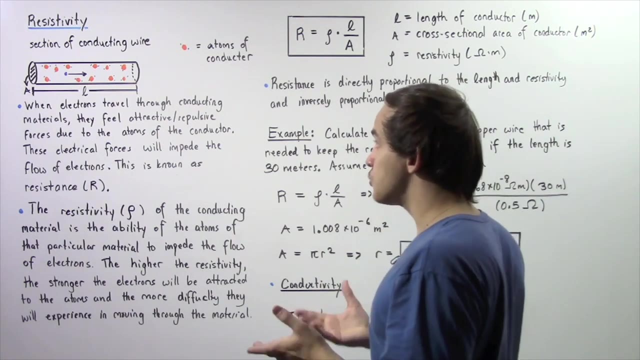 So let's actually discuss what takes place on the microscopic level when our single electron is traveling through our conducting wire, as shown. So let's suppose it's traveling in the positive direction along our x-axis. So these orange dots, along with the blue dots, are 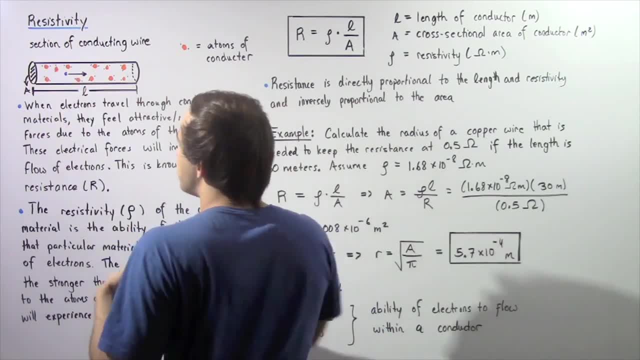 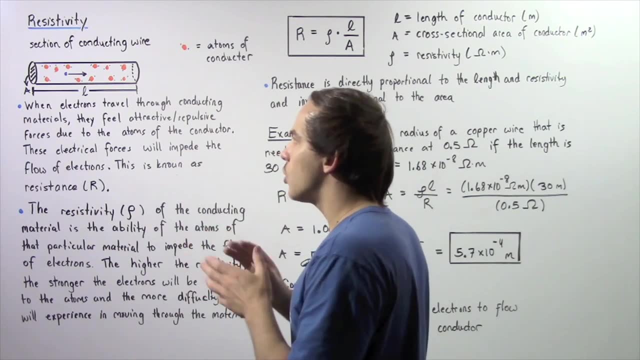 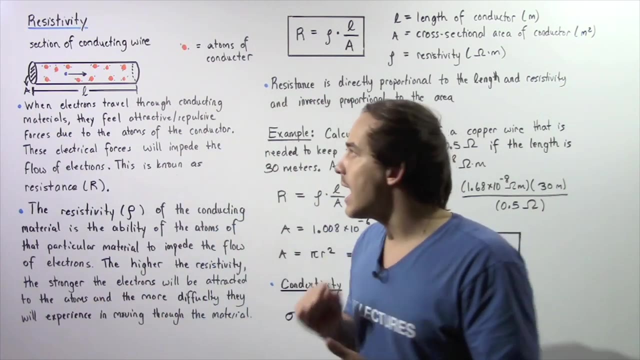 essentially the atoms of our conducting material. So we have the protons and neutrons found in the nuclei of the atom And we have the electrons which are orbiting those nuclei. Now, as you might know, atoms are mostly empty space And because the small size of our electron, this electron will have relative 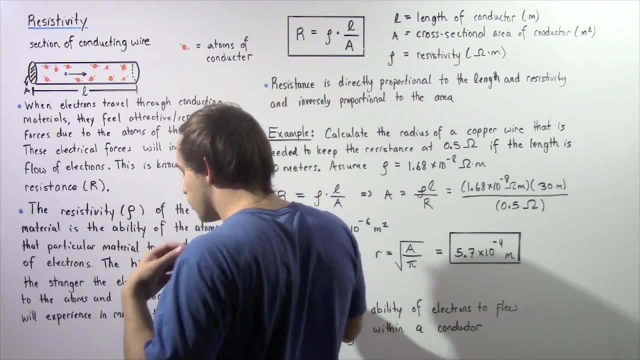 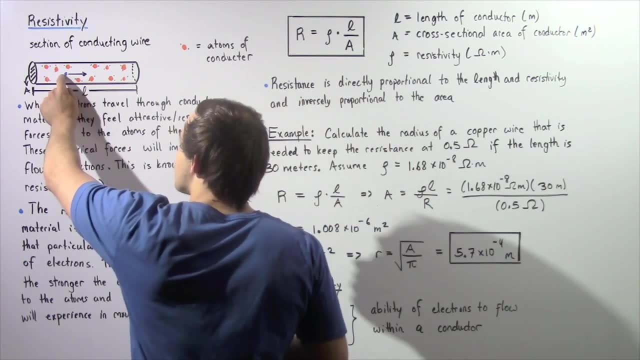 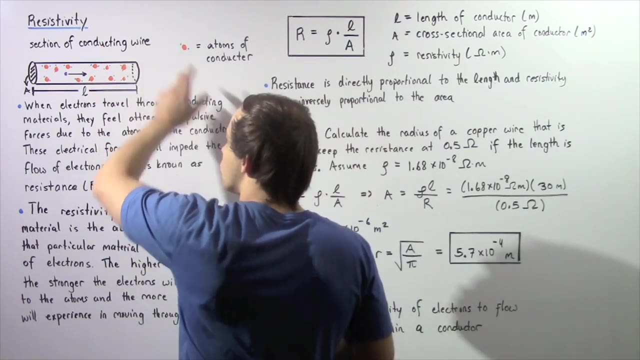 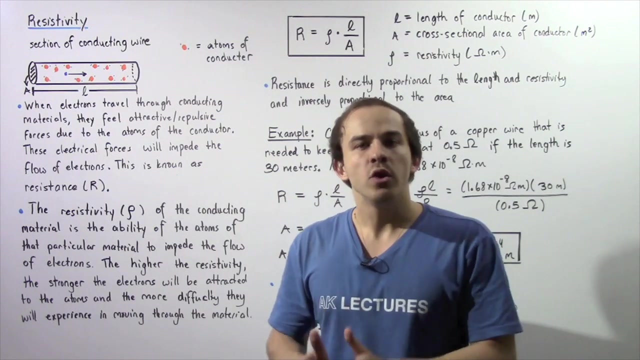 little difficulty in traveling through our conducting wire. However, it does experience difficulty, And that's because if this electron gets close to either the protons or the electrons of our conducting wire, then it will have relatively little difficulty in traveling through our conducting wire, Regardless of the atoms composing our conducting wire. attractive and repulsive. 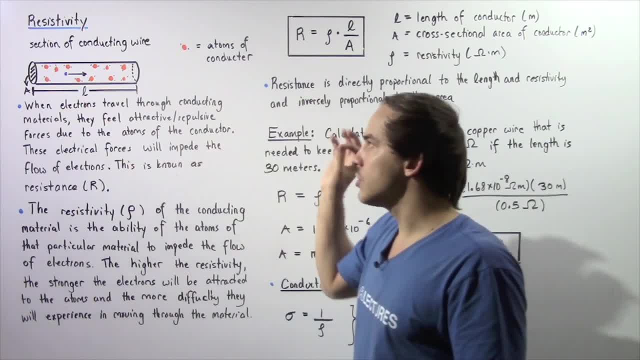 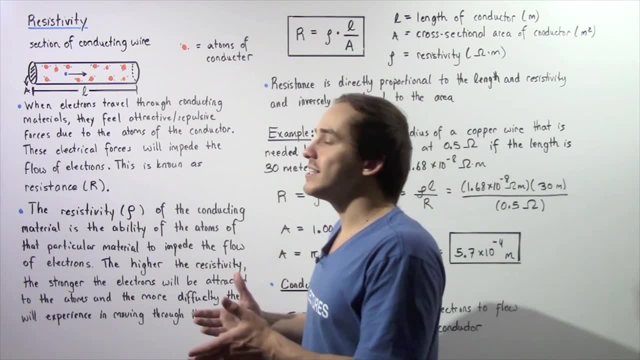 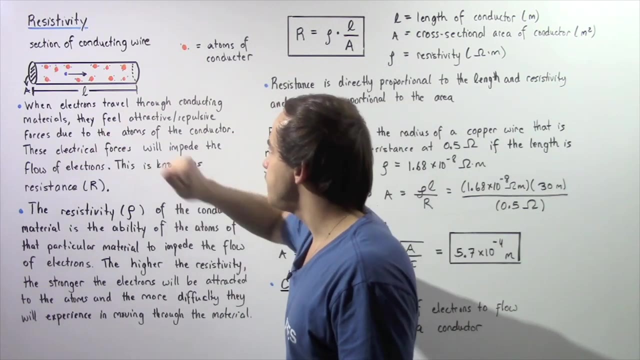 forces will be felt And these electrical forces will impede the flow of our electrons as it travels through our wire. So this effect, this impeding effect, is essentially known as resistance. If electrons travel through the particles they trap into the structure of the vielä-e electron. they try to make those electrons move with relative responds to the nope for a better effect. In other words, these electrons will be programmed into our conducting wire So this effective and title that are not regain visible will increase, whether one exposes the electrons or not. Let's suppose that the electrons travel down through our conducting wire, and they do this when our delicious ones, without a force on them, are login. So this impeding cuz therefore, in fact, is a matter that the electrons win over, And so here's a good line. 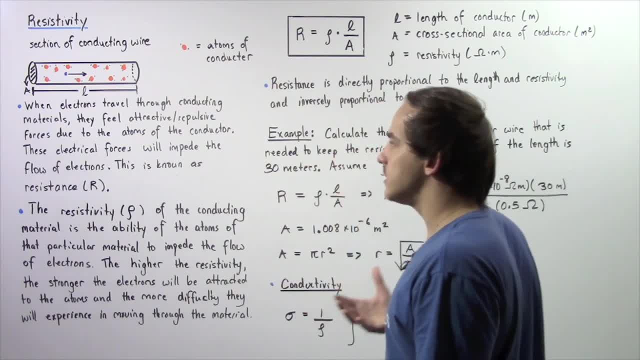 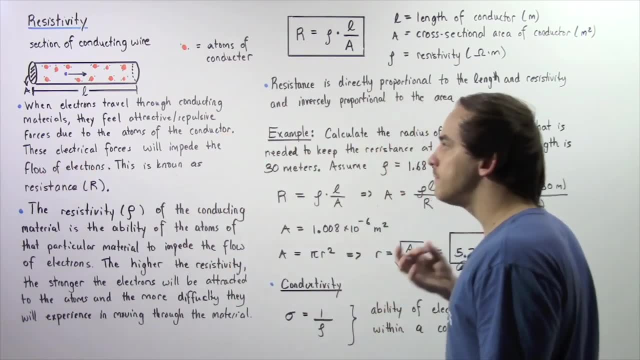 But the reason we're talking about electric economies is because electric scrutiny of nasıl we forces as a result of the atoms of our conducting material, so the protons and the electrons. Now these electrical forces will impede the flow of electrons and this concept is known. 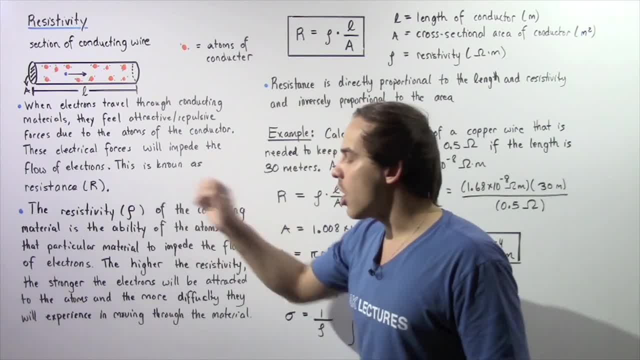 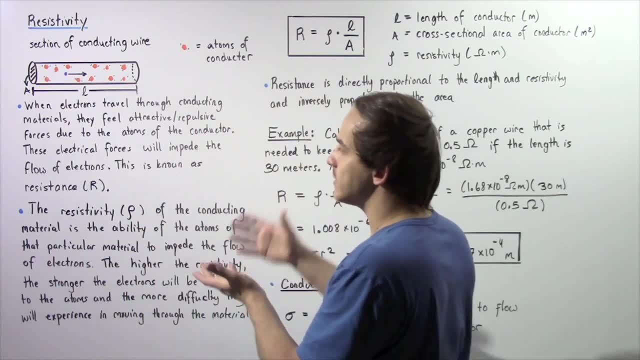 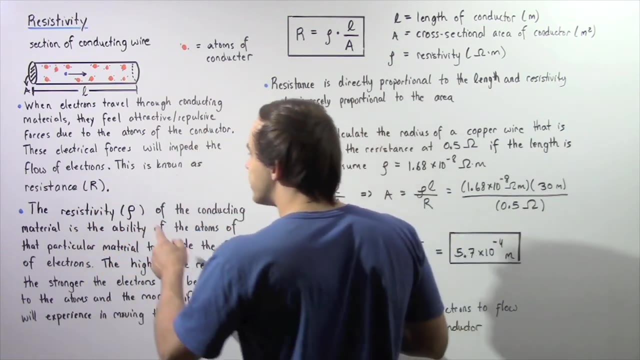 as resistance. It's given by a capital R. Now, resistance is not the same thing as resistivity, although these concepts are related, as we'll see in just a moment. So the resistivity of a conducting material given by the Greek letter Rho is the ability. 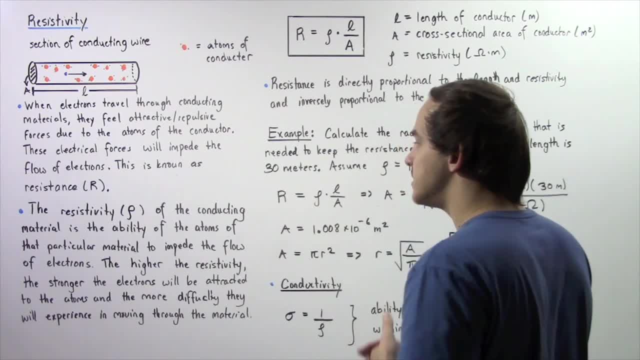 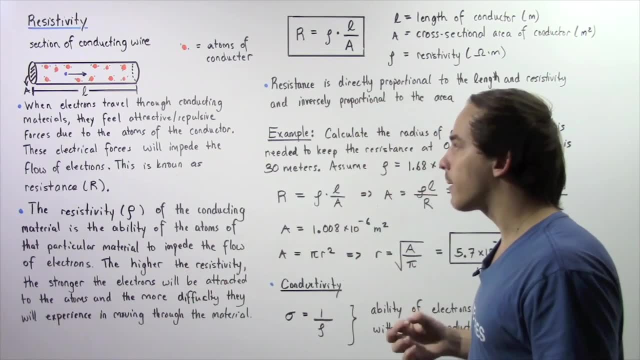 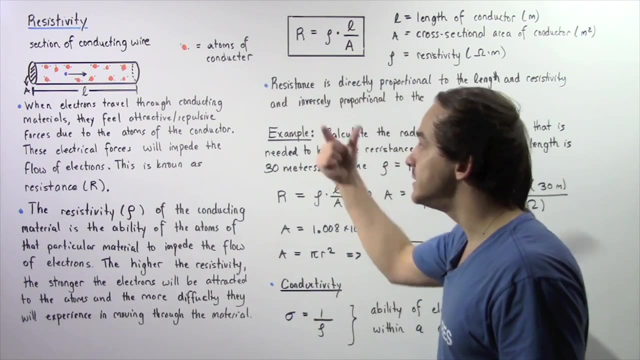 of the atoms of that particular conducting material to impede the flow of electrons. So the higher our resistivity of our particular material, the stronger the electrons will be attracted to the atoms of that material and the more difficulty those electrons will experience in moving. 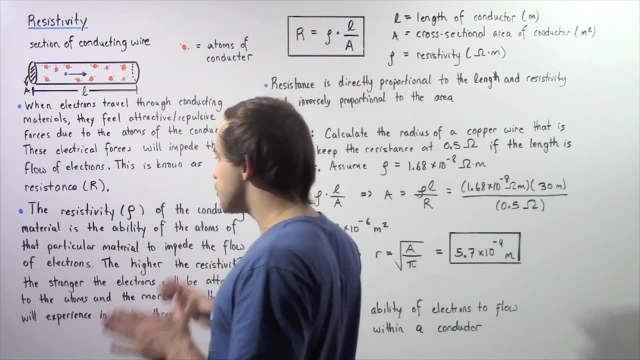 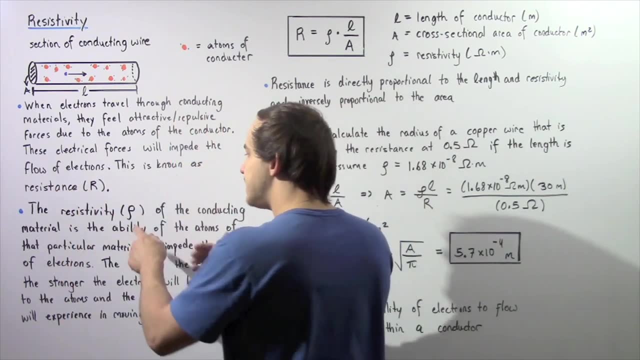 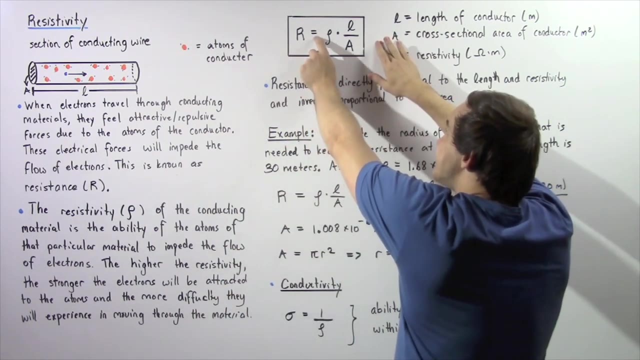 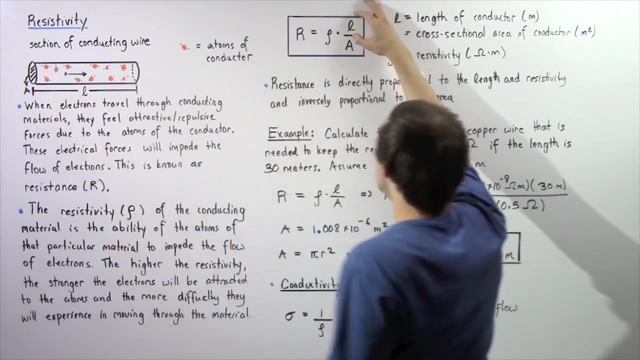 through that particular conducting wire. So what exactly is the relationship between resistance given by R and resistivity given by Rho? So it's given by the following equation: Our resistance given by R is equal to the product of Rho, our resistivity multiplied by the length of our wire. 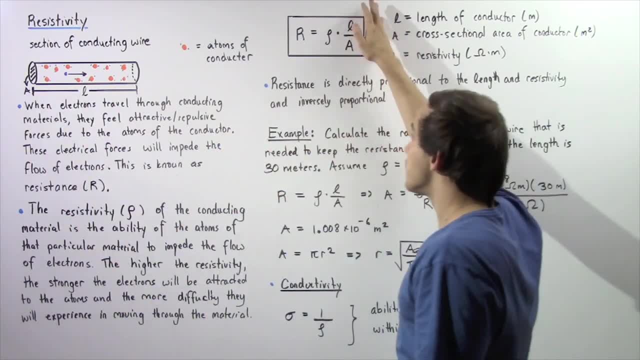 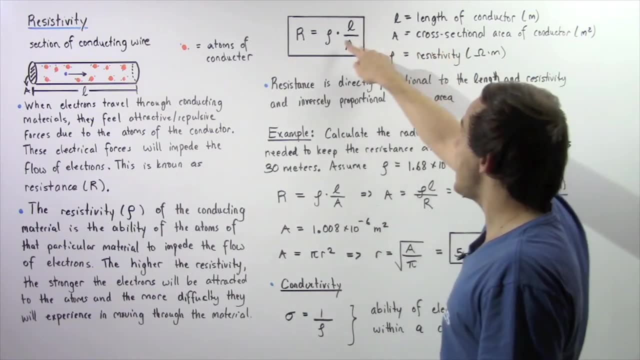 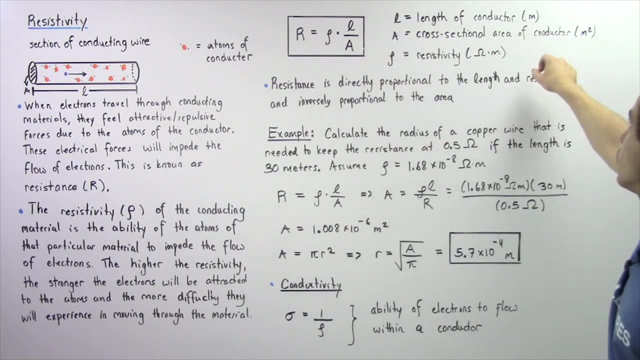 divided by the cross-sectional area of that wire. So once again, our Rho is the resistivity. It has units omega multiplied by meters. The A is the cross-sectional area of the conducting wire given by meters squared, and the L is the length of the conductor wire given by meters. So we see: 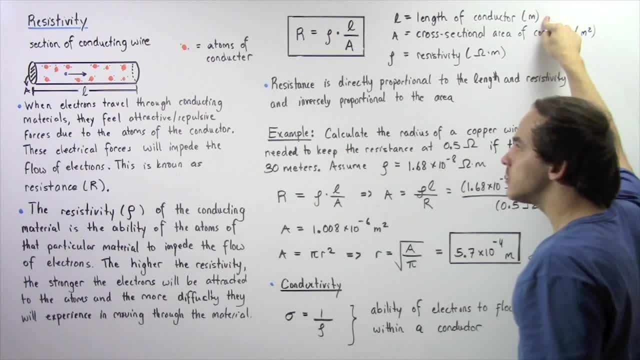 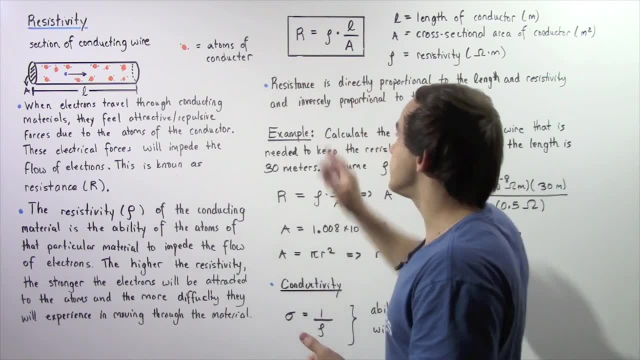 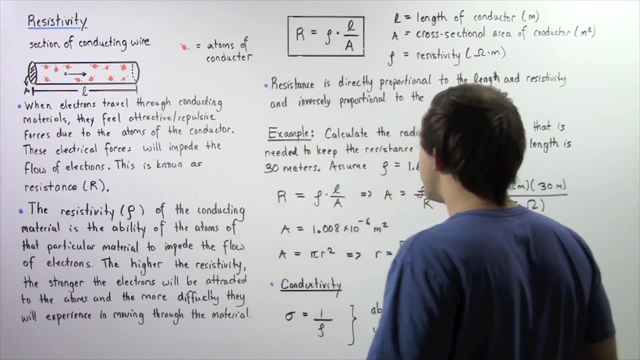 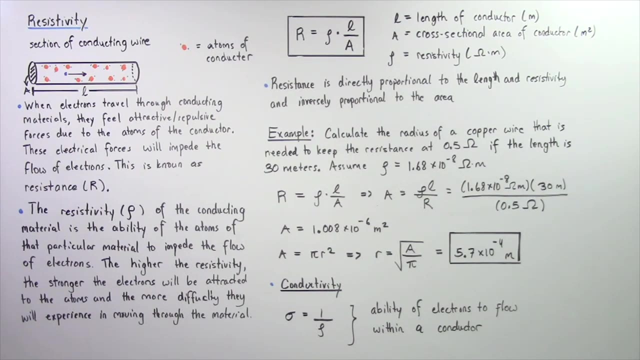 atoms of the material to attract that electron, and so our resistance will increase. So let's look at the following example in which we're going to apply this equation: Calculate the radius of a copper wire that is needed to keep the resistance at 0.5 ohms. 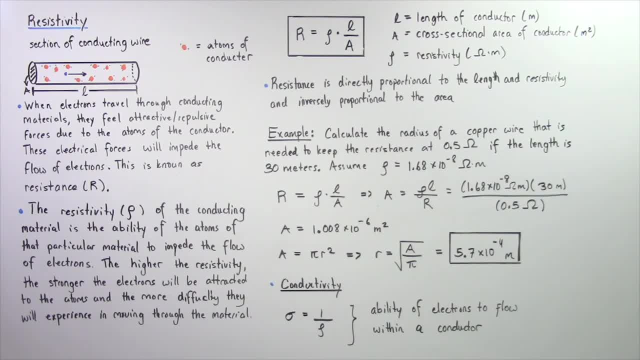 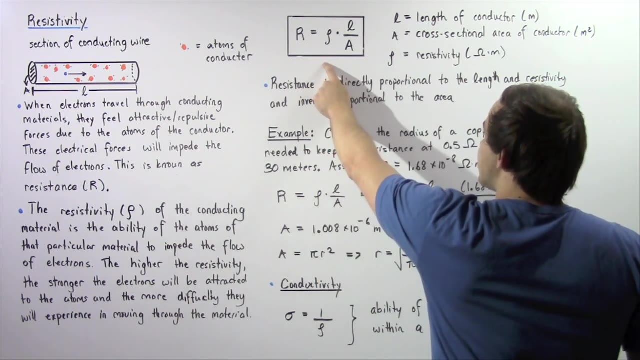 if the length of the wire is 30 meters, Assume that our resistivity of the copper is given to be 1.68 times 10 to the negative date omega multiplied by meters. So we begin with this equation. We have to rearrange it and solve for our A. The A is equal to the product of this quantity. 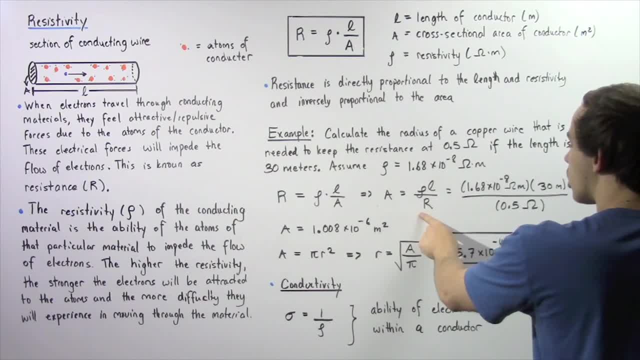 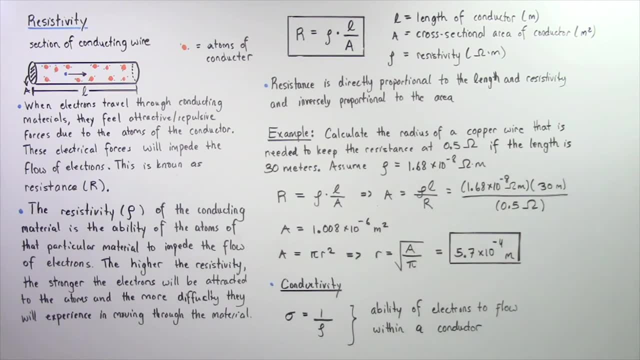 our rho multiplied by L, divided by our R. So our rho is this quantity: Our length is 30 meters and our R is 0.5 ohms. We multiply, divide and we get 1.008 times 10 to the negative date omega, multiplied by. 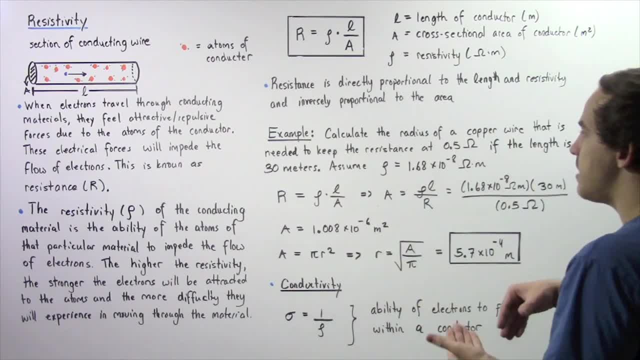 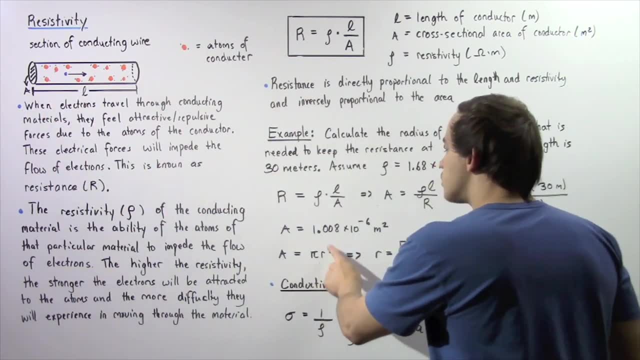 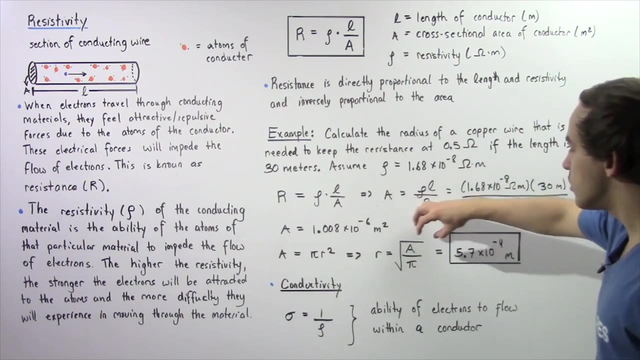 6 meters squared. So we're going to make the assumption that our wire is cylindrical. So that means the area is given by pi R squared. So we take this, solve for our R. We see the R is equal to the square root of the ratio. 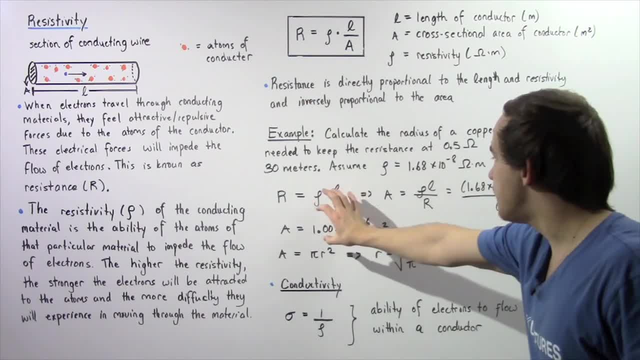 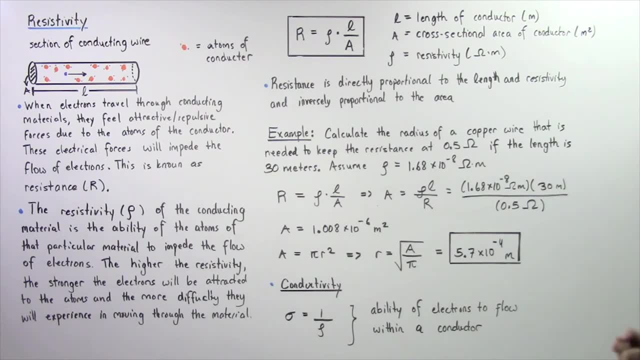 of the area to pi. So the area was found in this part. We plug that in and we solved and we get about 5.7 times 10 to the negative 4 meters. This is the radius of our conducting wire. Now, before we end this lecture, let's discuss one other concept. 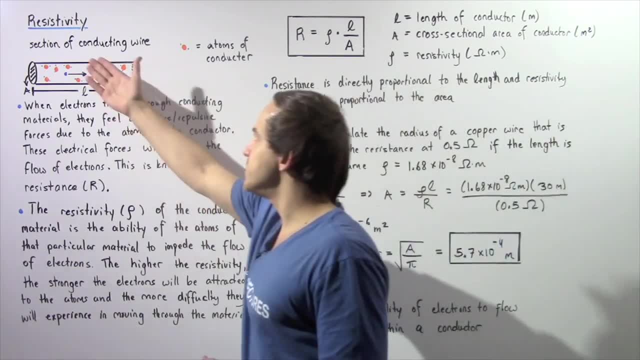 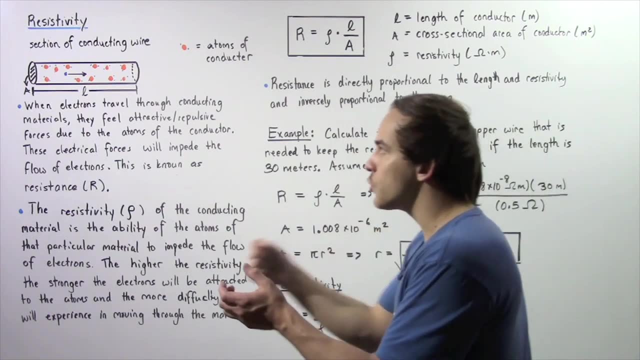 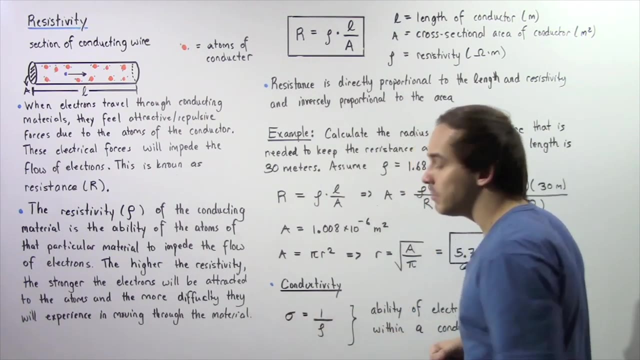 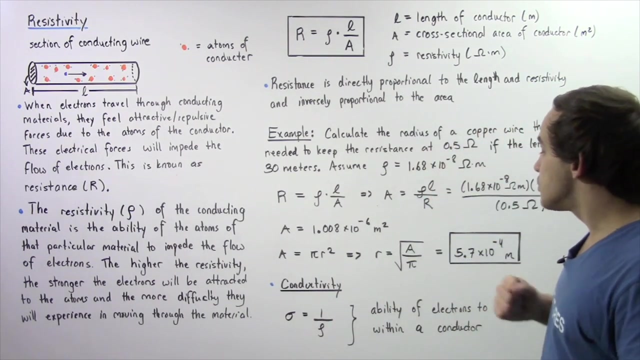 So this concept is essentially the opposite of resistivity. So this is known as conductivity. It's essentially the ability of the atoms to flow through our wire freely. So the conductivity of a material is given by the Greek symbol sigma, And sigma is equal to 1 divided by our resistivity, given by rho. 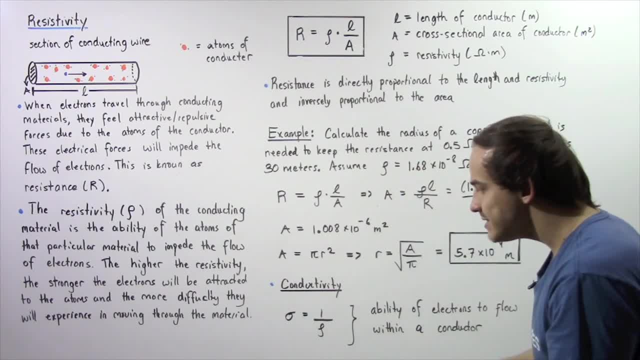 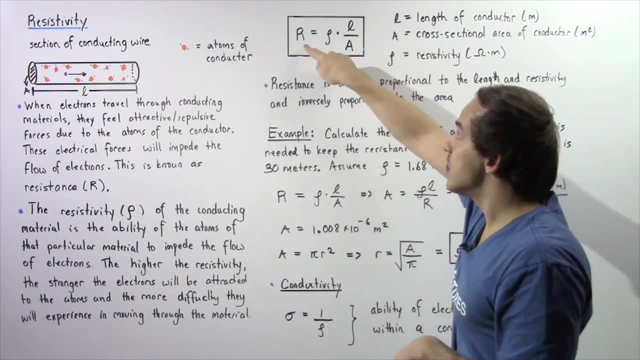 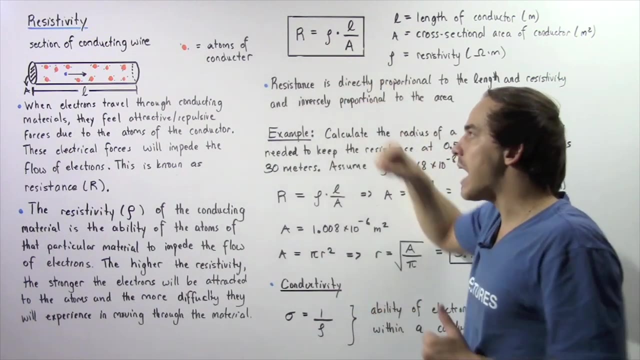 So we see that if our resistivity decreases, that means our conductivity increases, And that makes sense, because if this decreases, the resistance decreases and that implies that the electrons are able to flow more freely through our conducting material. So, once again, this is simply the ability of the electrons to flow. 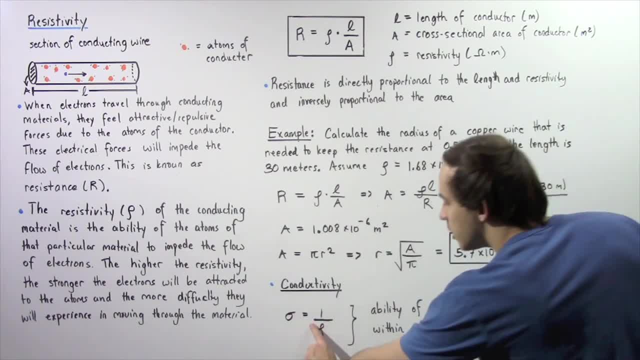 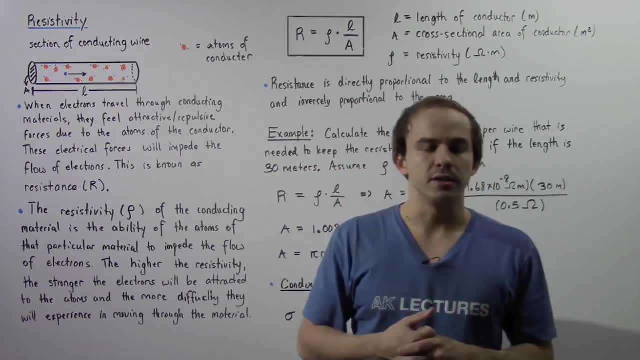 Within our conductor, The higher this value is. the lower this value is and the more able our electrons are to flow through that conducting material.